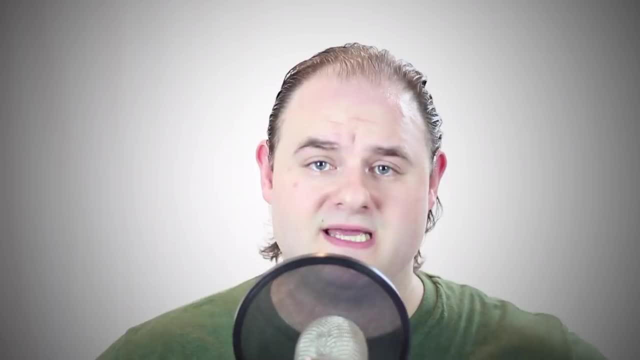 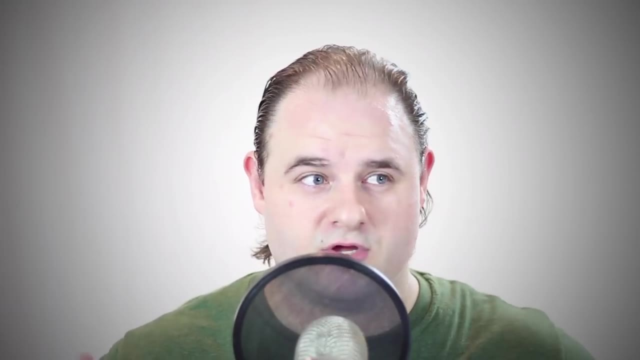 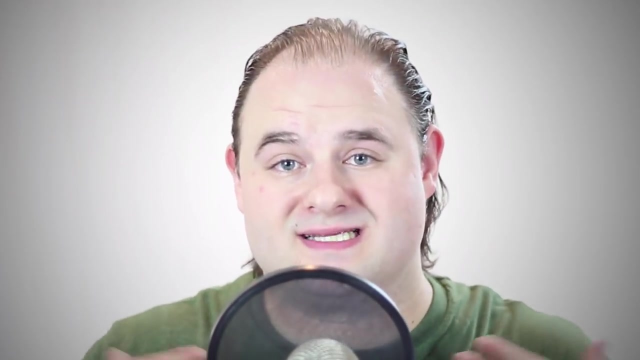 keep in mind: if you do record your brainstorming session, somebody is going to have to go back and notate everything, So you could also try to use some kind of notation software, but that can be a little wonky at times, So this is why we decide to use Google Docs. The thing is, 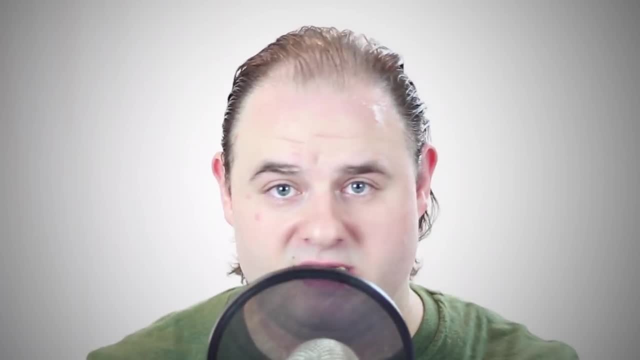 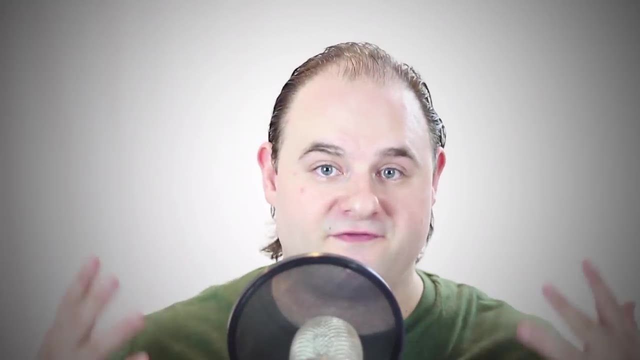 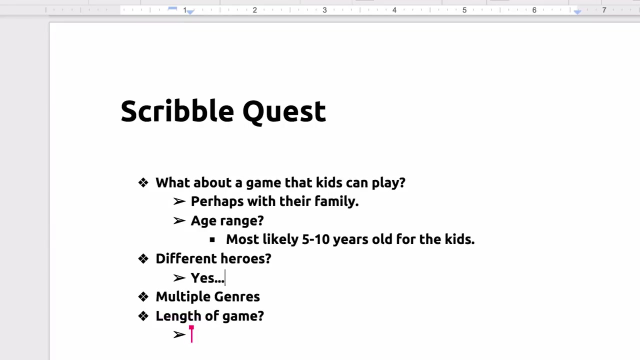 we can share it while we work, it saves automatically and we can go back to it whenever we need to. Now, all we're doing here is just proposing ideas, little what-if scenarios. We propose an idea, this makes us ask a question, and then we answer that idea, which again generates. 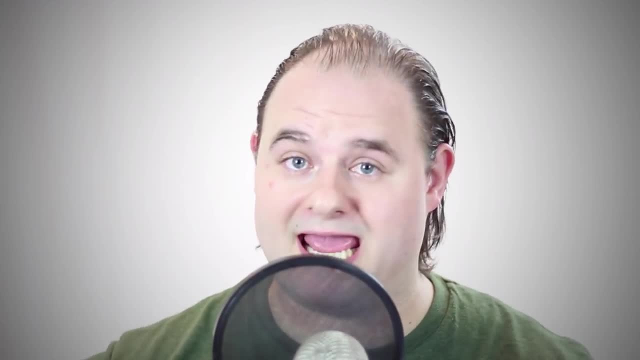 another question: Okay, now that we have a bunch of ideas, we're going to start handling them. So, we're going to start handling them. Okay, now that we have a bunch of ideas, we're going to start handling them. Okay, now that we have a bunch of ideas, we're going to start handling them. 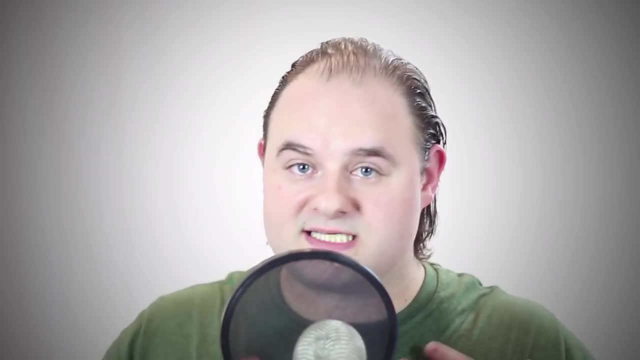 Okay, now that we have a bunch of ideas, we're going to start handling them. Right now, we're just hammering these ideas down. Now, what has worked for myself and my team is that we use the Think and Wait method. This is essentially 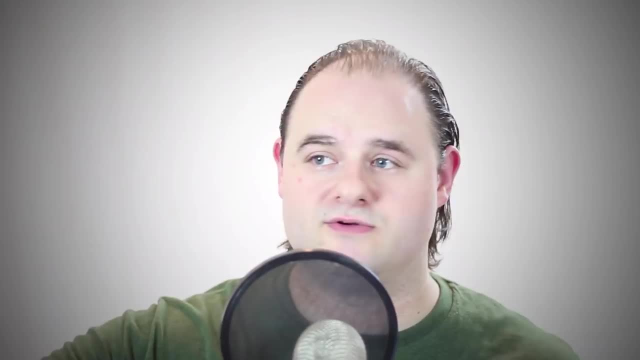 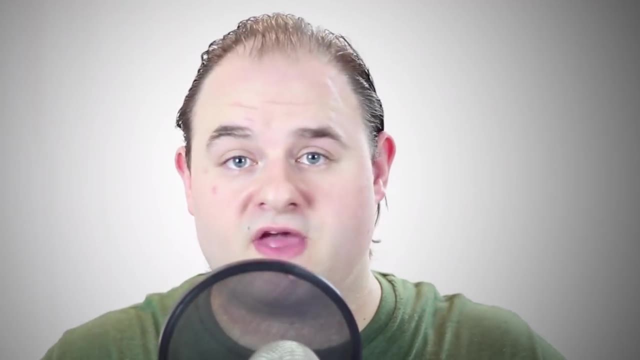 we give the brainstorming session a day or two to kind of mature, and then we come back to it and look at it with fresh eyes. I use the Think and Wait method with our board game, The Quest for Runeum. It takes time, but again I found it. the. 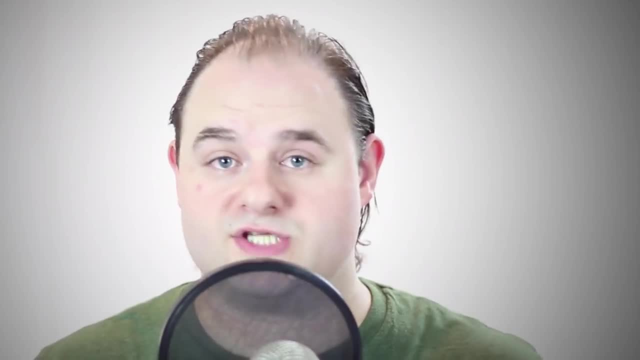 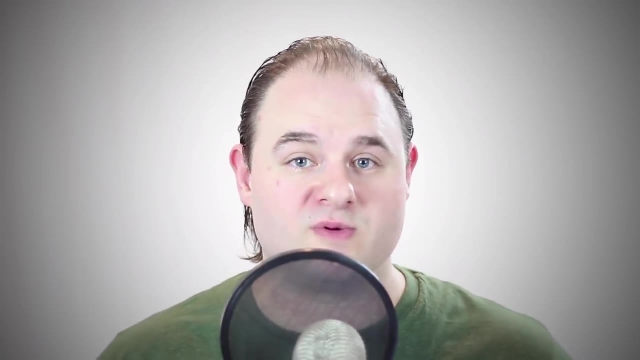 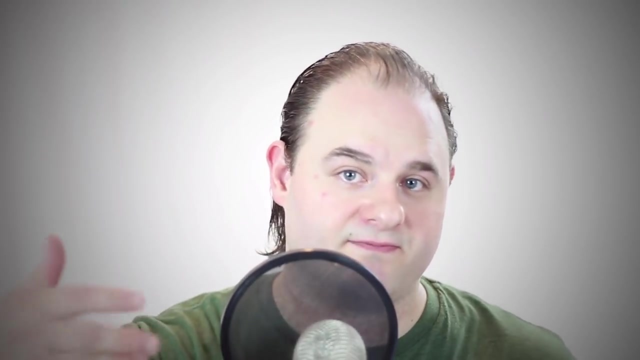 most effective, especially when I was a solo team few years ago. so after we brainstorm, we decided to do another brainstorming session now. the one that you saw was actually session number two, and at that point we were naturally beginning to go into the concept phase. the concept phase simply means that we're beginning to make decisions. 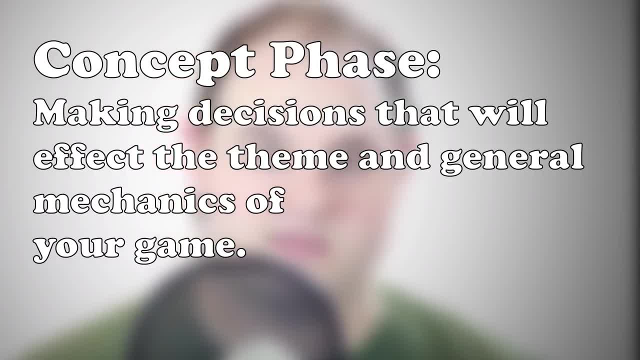 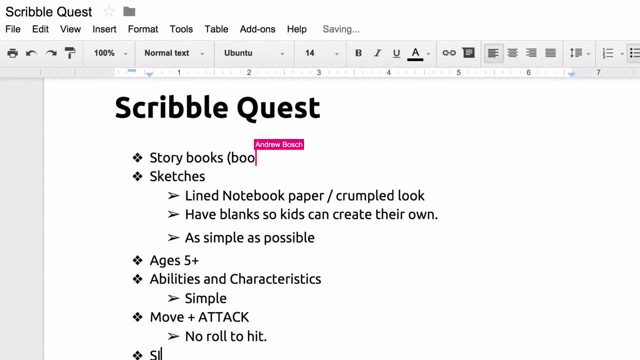 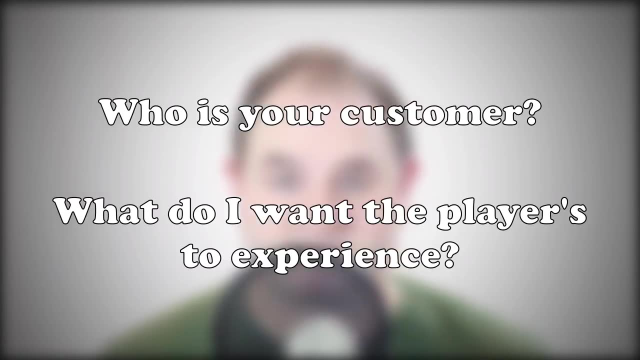 that's affecting the general theme and mechanics of the game, so we're actually using the same document that we used before. the concept phase is all about the two most important questions: who is your customer and what do i want the players to experience when you begin answering? 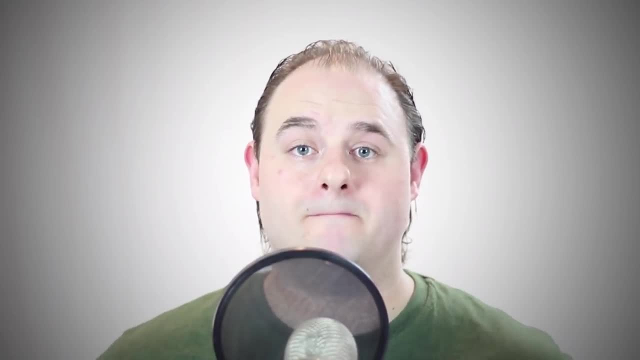 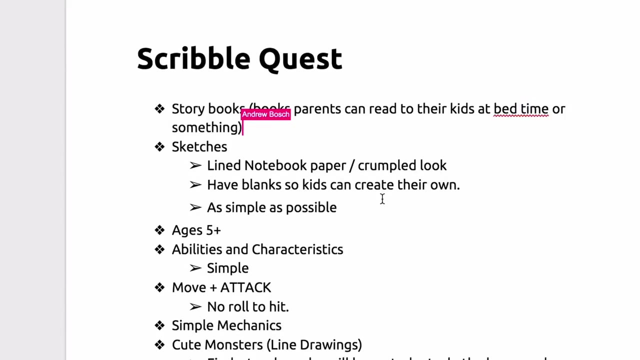 these important questions. they're going to spur more questions which you're then going to want to answer. now you may not be able to answer all these questions quite yet, but the more that you can nail down, the better it's going to be in the next stage of creating your board game.